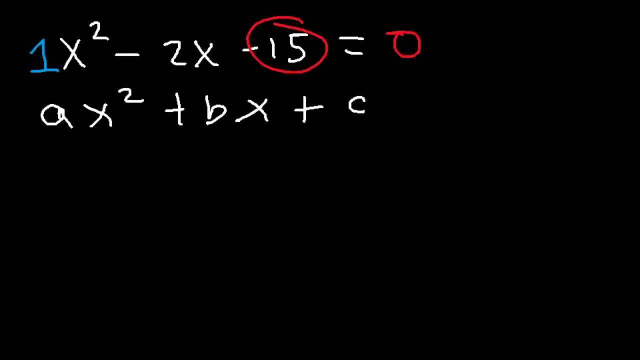 And c is the number that doesn't have an x attached to it, So c is negative 15.. So let's go ahead and write that. So a is 1., b is negative 2. And c is negative 15.. Now here's the quadratic formula: x is equal to negative b plus or minus the square root. 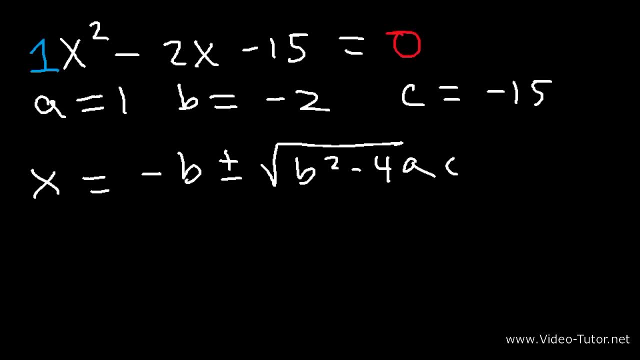 of b squared minus 4ac divided by 2a. So let's go ahead and plug in the numbers that we have. So b is negative, 2. b squared: Negative 2 squared, That's negative 2 times negative, 2. That's positive 4.. 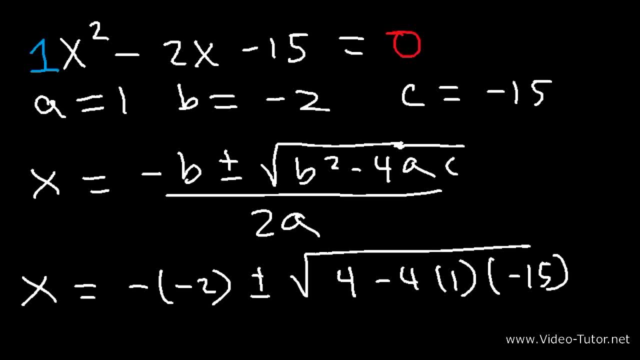 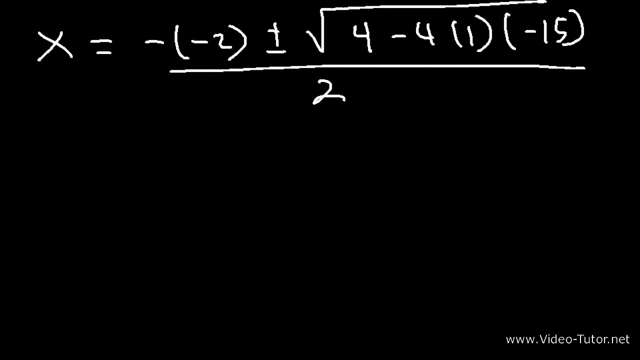 a is 1. And c is negative 15.. Divided by 2a or 2 times 1,, which is 2.. Now let's go ahead and simplify this result: Negative times negative. 2 is positive 2.. 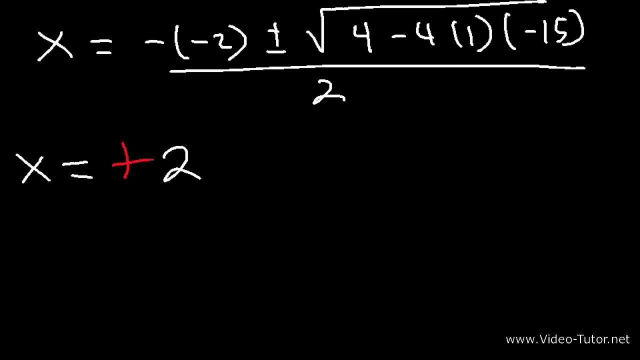 Negative times negative, 2 is positive 2.. On the inside we have negative 4x Negative 4 times negative, 15. That's positive 60. So this is going to be plus or minus square root 4 plus 60 divided by 2.. 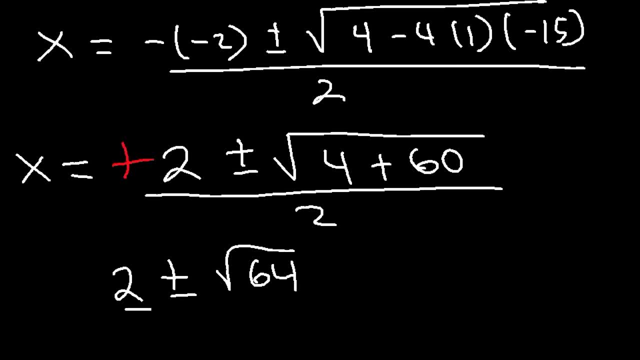 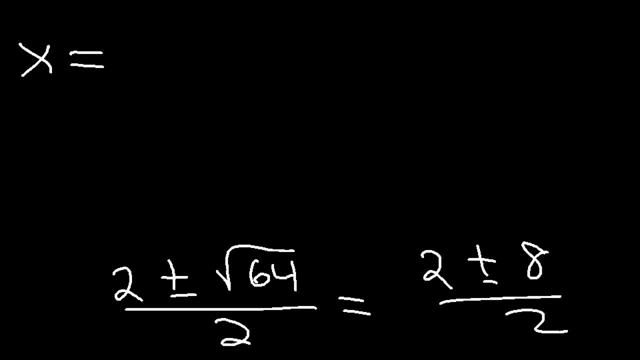 this point we need to separate into two answers. notice that we have the symbol plus or minus, so it's going to be 2 plus 8 divided by 2, and the other answer is 2 minus 8 divided by 2. 2 plus 8 is 10, and 10 divided by 2 is equal to 5. now 2. 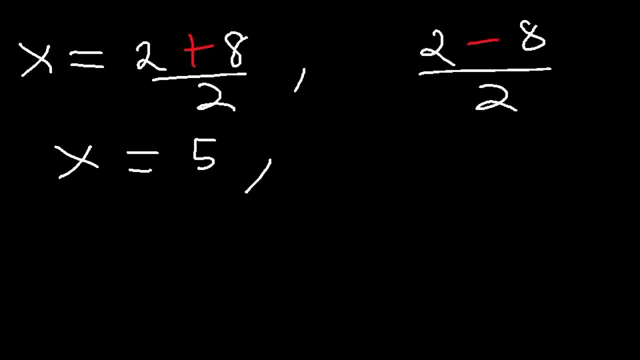 minus 8 is negative 6, and negative 6 divided by 2 is negative 3. so these are the two answers and that's how you can use the quadratic formula in order to solve quadratic equations. but for the sake of practice, let's go ahead and work. 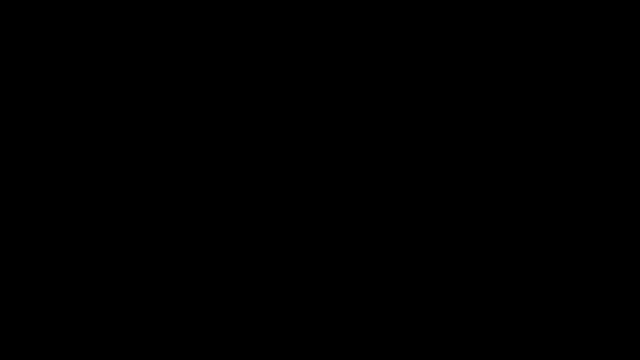 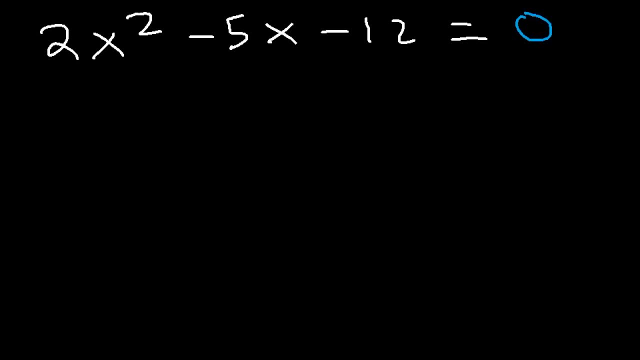 quadratic formula to get two solutions for this equation. so let's identify a, B and C. a is equal to 2, B is negative 5 and C is equal to negative 12. so, using the quadratic equation, X is equal to negative B. so B is negative 5 plus or. 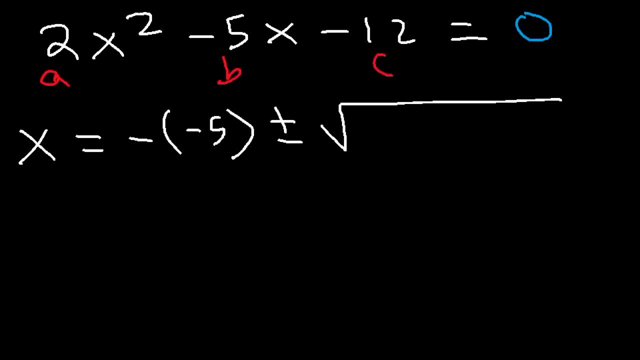 minus square root, B squared negative 5 squared is positive 25 minus 4 times a, which is 2 times C, which is negative 12 divided by 2a. so negative times negative 5 is positive: 5: 2 times 12 is 24. 4 times 24 is 96. now, because we have two negative signs, it's 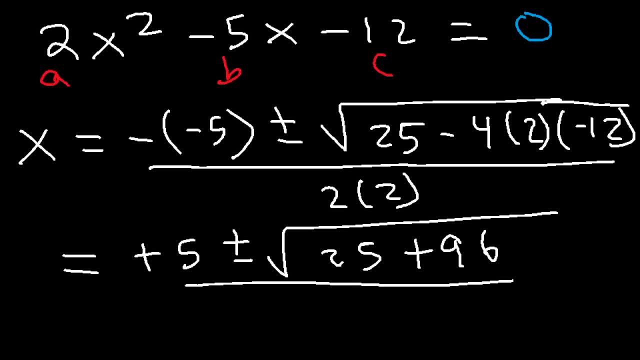 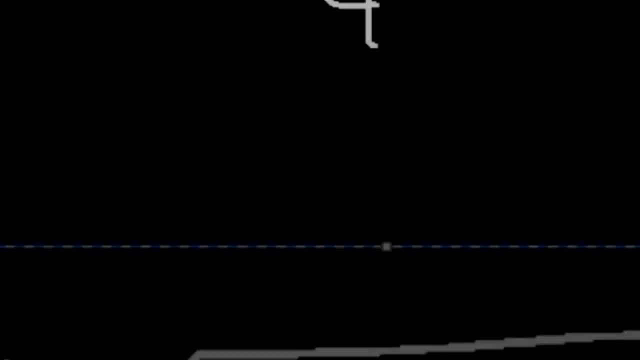 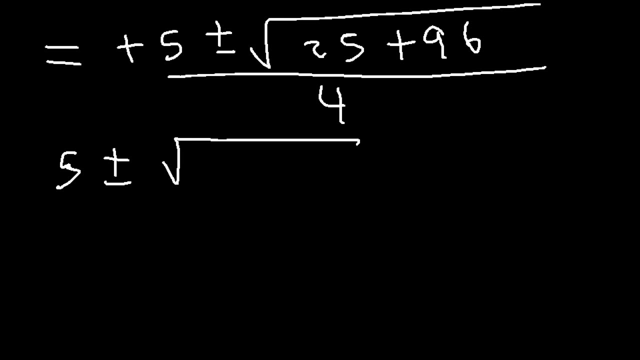 going to be positive. 96 divided by 2 times 2, which is 4. now, what is 25 plus 96? how much is that? well, 90 plus 20 is 110. 5 plus 6 is 11. 110 plus 11 is 121, and the square root of 121 is: 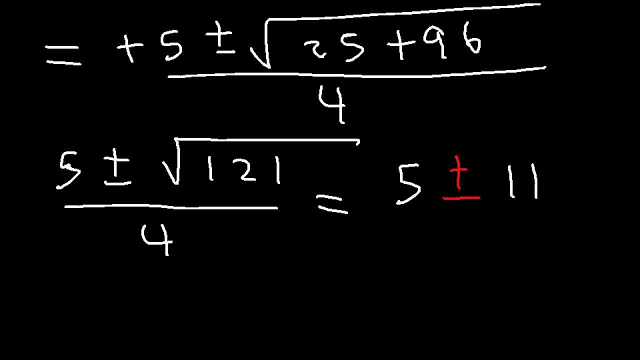 11. so we have 5 plus or minus 11 divided by 4. so now what we're going to do is write two equations. the first one is going to be 5 plus 11 over 4, and the second one 5 minus 11 over 4. 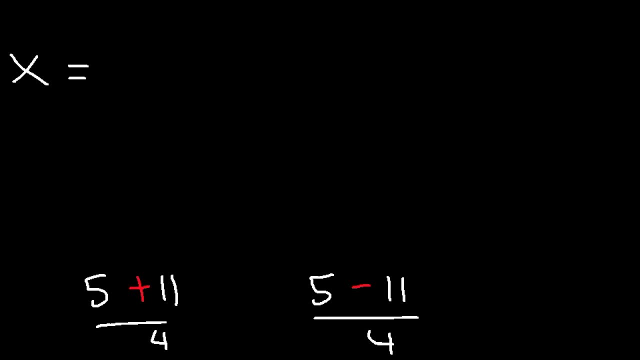 now, 5 plus 11 is 16 and 5 minus 11 is negative. 616 divided by 4 is 4. negative 6 divided by 2, we can reduce it. both numbers are even. so we can divide by 2. negative 6 divided by 2 is negative. 3. 4 divided by 2 is 2, so X is equal to. 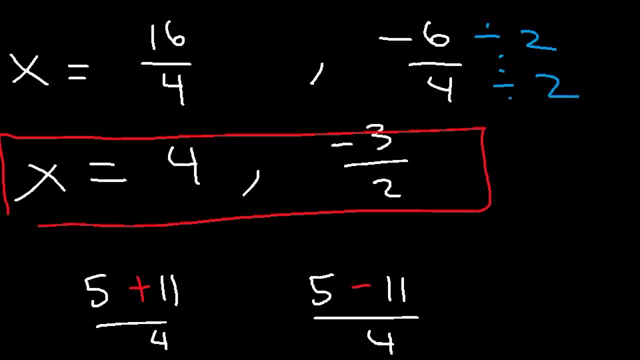 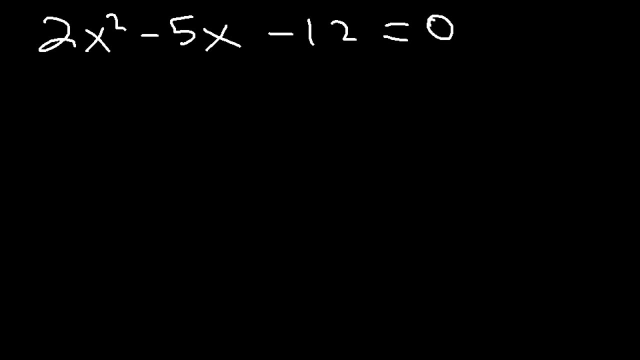 4 and X is equal to negative 3 over 2. so that's the solution to the equation. now let's go back to our original equation, which was 2x squared minus 5x minus 12, because you can also solve this equation by factoring. however, sometimes some 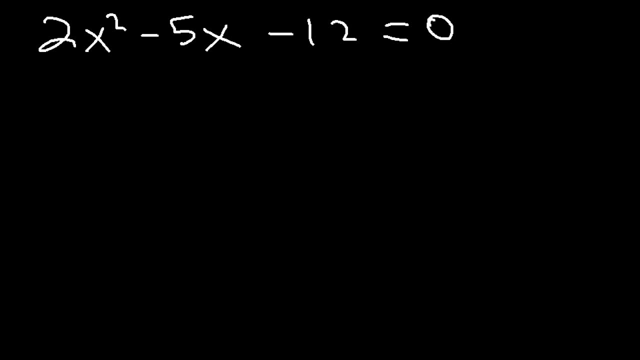 equations might be difficult to factor. let's say, if you have an equation that's factorable but it's very difficult to factor, how can you factor? well, you can use the quadratic formula. let's use this as an example. so we know that everything is equal to zero. so we can use this as an example. so we know that. 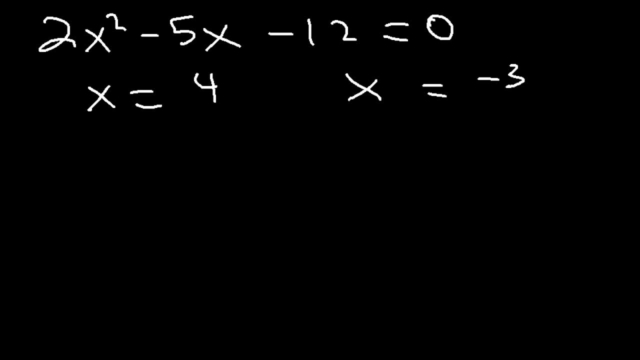 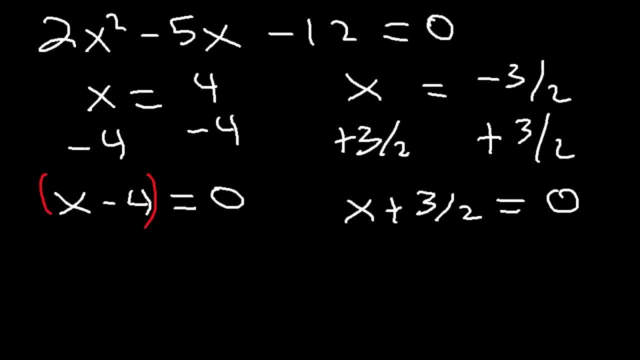 Now, since we have a fraction, what we want to do is multiply both sides of the equation by 2 to get rid of the fraction. So 2 times x is 2x, 2 times 3 over 2, the 2's will cancel and you're going to get 3.. 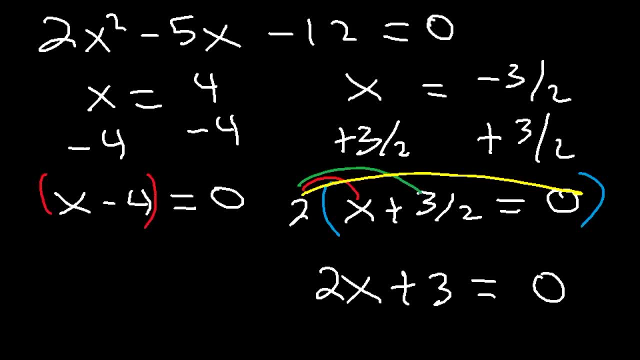 And finally, 2 times 0 is simply 0. So this is another factor. Therefore, to factor the expression 2x squared minus 5x minus 12, it's going to be 2x plus 3 times x minus 4.. 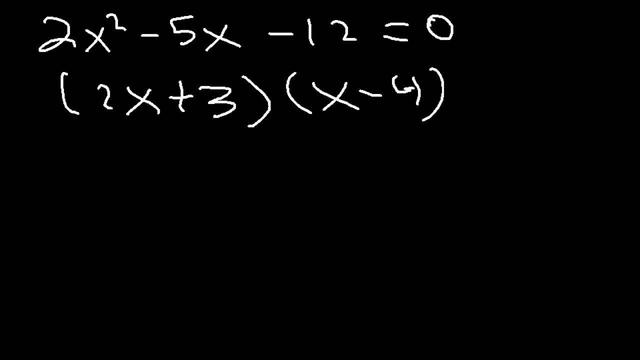 Now we can check the work. You can check the answer by FOILing it, So let's go ahead and do that. 2x times x is 2x squared. 2x times negative: 4 is negative 8x. 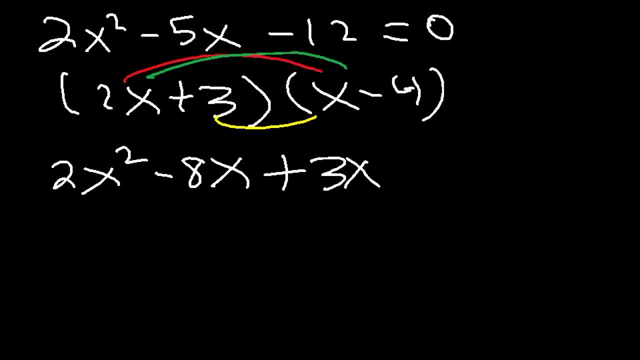 3 times x is 2x, squared. 2x times negative, 4 is negative 8x. 3 times x is 3x and 3 times negative, 4 is negative 12.. And now let's add the two like terms in the middle. 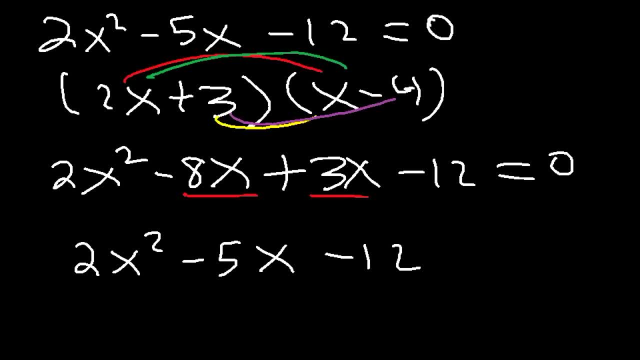 Negative. 8 plus 3 is negative 5.. So notice that we do indeed get the original equation. So if you ever need to factor a trinomial, you can always use the quadratic formula to factor it. If you ever have difficulty factoring a difficult expression, you can always use the quadratic. 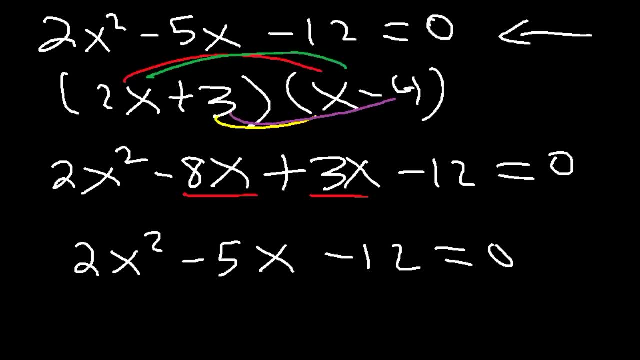 formula to factor it. If you ever have difficulty factoring a difficult expression, you can always use the quadratic formula to factor it. This is very useful. But now how can we actually factor this particular trinomial where the leading coefficient is not 1?? 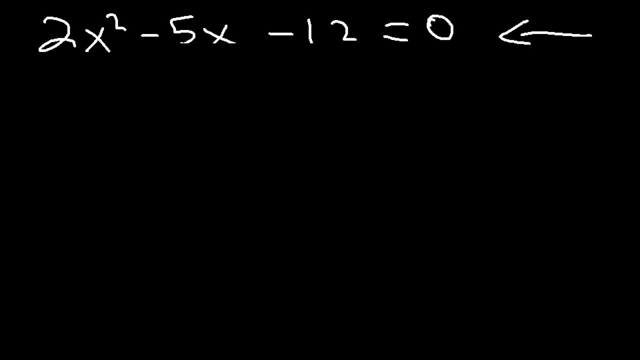 What's the standard way of doing it? The first thing that we need to do to factor this expression is we need to multiply the leading coefficient by the constant term. So 2 times negative 12 is negative 24.. Now ask yourself what two numbers multiply to negative 24. but add to the middle coefficient. 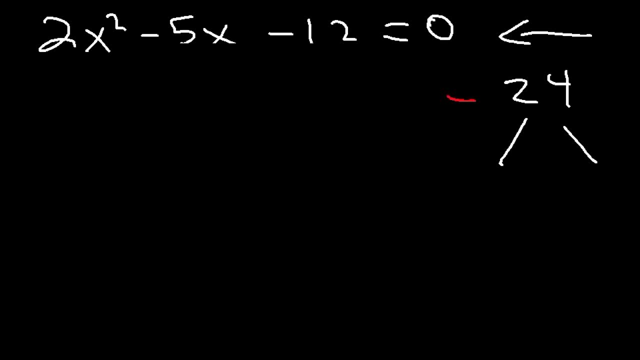 3., 4., 6., 7., 8., 9., 10., 12., 4., 12., 1.. Now here's the first thing you need to do: to calculate the substitution of negative 5.. 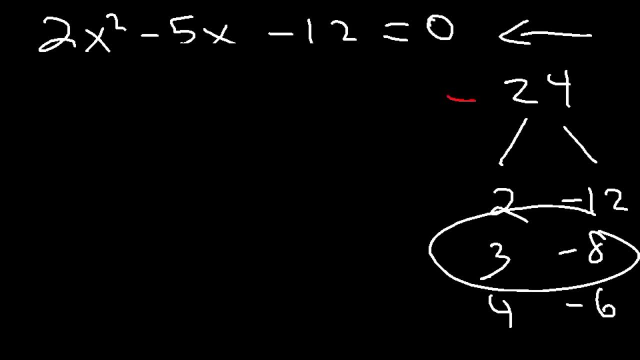 Now you might be thinking a list of answers. We have 2 and negative 12.. 3 and negative 8.. 4 and negative 6.. But notice that 3 and negative 8 differs by negative 8, I mean not negative 8, but 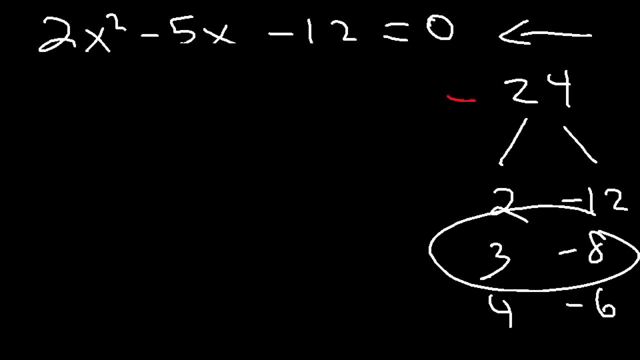 negative 5.. 3 plus negative 8 is negative 5.. So what we're going to do at this point is we're going to replace negative 5x with a negative 4x, And so we're going to take 8 minus 5x. and we're going to take 8 minus 5x, and that's. 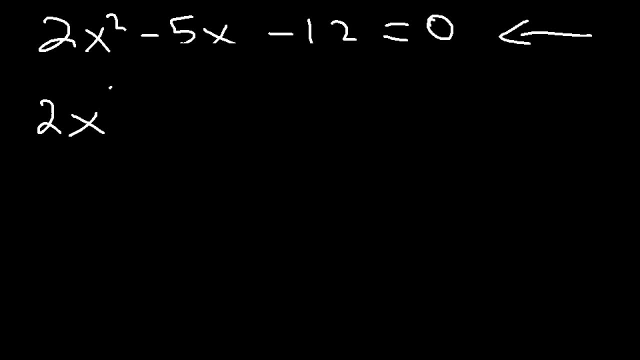 the equation. So 1 plus 8 is negative 5x, with negative 8x and positive 3x. The order doesn't matter, but I just prefer to put the even numbers next to each other. Now, in the next step, we're going to factor by grouping. 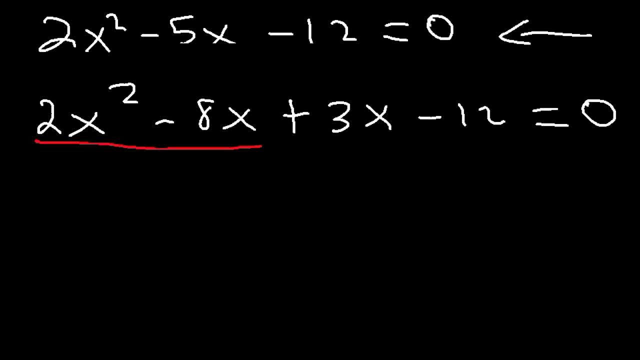 In the first two terms. take out the GCF. The greatest common factor between 2 and 8 is 2.. The greatest common factor between x squared and x is simply x. 2x squared divided by 2x is equal to x.